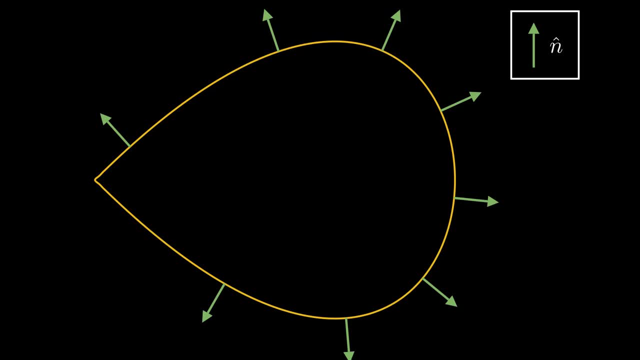 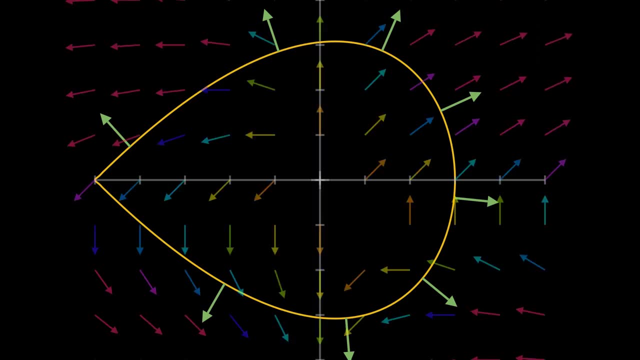 You can see how the vectors are always perpendicular to the curve In a two dimensional context. the goal of the flux integral is to measure the flow rate through a curve. How would we measure this? As with most calculus topics, let's try to zoom into the curve. 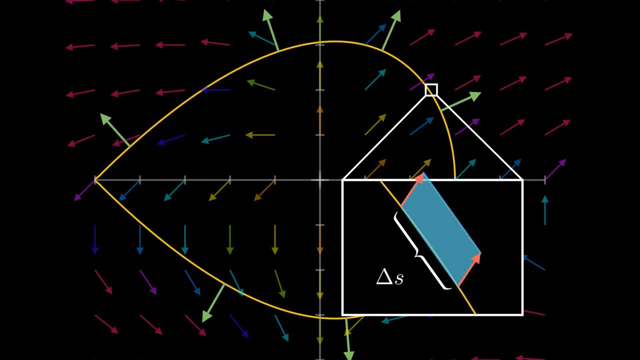 making it almost like a straight line. If we can measure the flow rate of this small piece of the curve, we can measure the flow rate of the entire curve through an integral over the curve, Similar to a lot of topics in vector calculus. it's easier to understand. 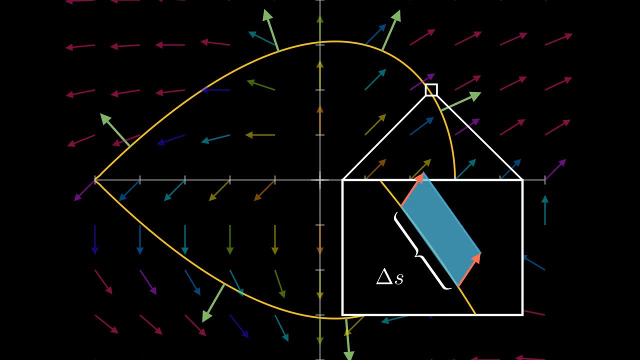 topics when we think about the vector field showing some sort of fluid, some incompressible fluid like water. So, for a small change in time, which I'll call delta t, the amount of fluid passing through the segment delta s can be measured by this parallelogram. 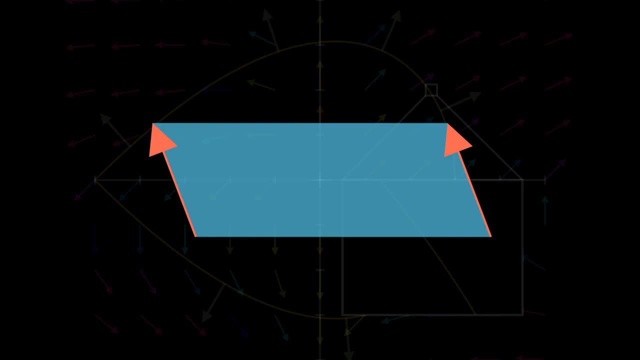 Now let's take a closer look. As you know, the area of a parallelogram is simply the base times the height. Well, the base of this parallelogram is delta s and the height of the parallelogram is the component. 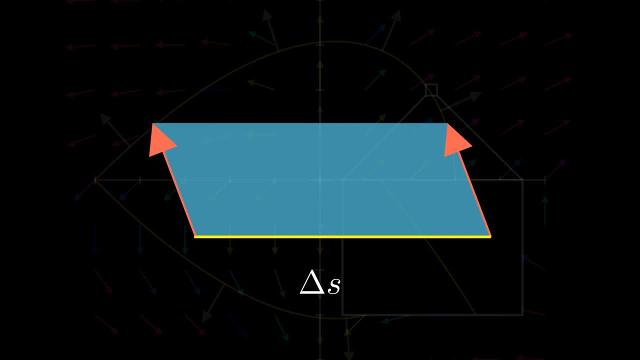 of our vector function at time t, perpendicular to delta s. It sounds a bit confusing, but essentially we're looking at the magnitude of this vector, which you can see is perpendicular to delta s. This is where we use n-hat To get the height of the parallelogram. we simply take the dot. 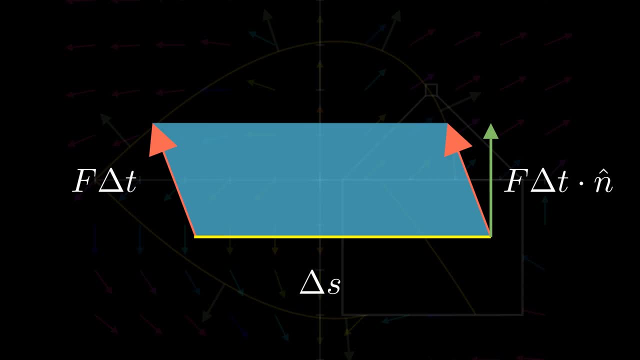 product between our vector field f and n-hat and multiply it by delta t. So the area of one parallelogram is f? dot n-hat times delta t times delta s, ie the flow through this parallelogram is f? dot n-hat times delta t times delta s. 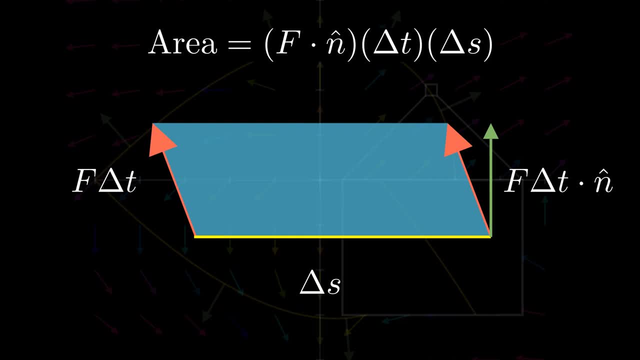 Now what we want is the area per unit time, which is the flow rate. So to find this in the graph, we divide it by delta t and we get that f dot n-hat times delta s. And finally, to measure the rate of flow through the whole curve, we just need to integrate. 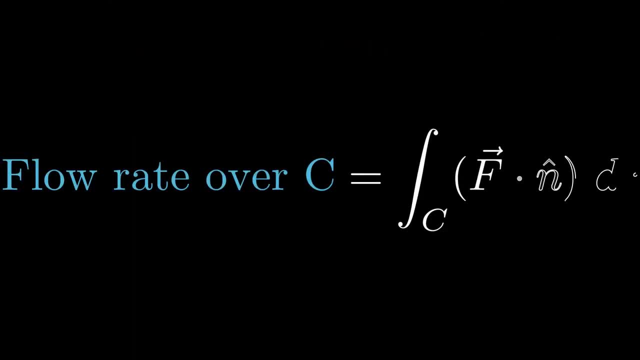 over the curve. This is just a line integral. thus our flux integral looks like this: this integral over c of f, dot, n-hat times s. This is the flow rate. You can see that we almost got this, so we'll just divide it by. 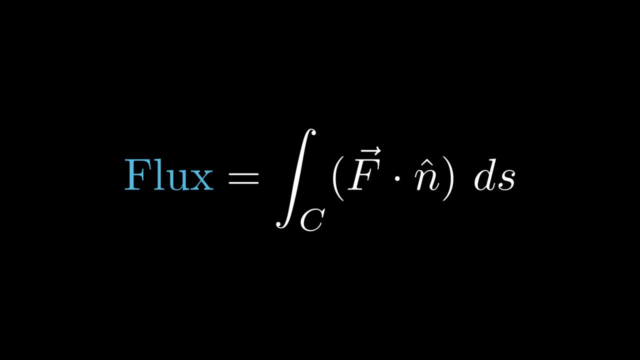 delta t and get f dot n-hat times delta s To measure the rate of flow through the whole. And there's a good chance you've heard this term, flux, before. Specifically, you might have heard of electric flux or magnetic flux. It's more common that you see these terms. 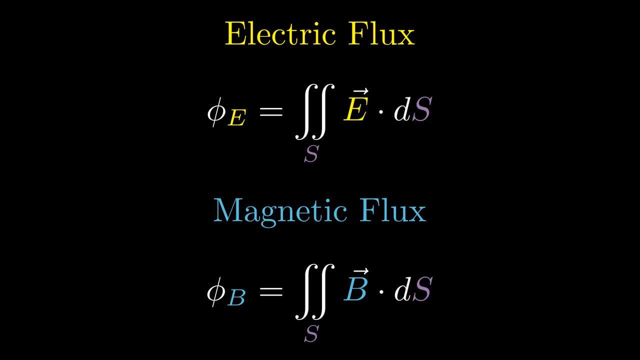 being used in 3 dimensions, where the flux integral just measures the flow rate through a surface. A flux integral in 3 dimensions is a similar concept, but instead of integrating over a curve, we are integrating over a surface, That is, we are finding the flow rate through. 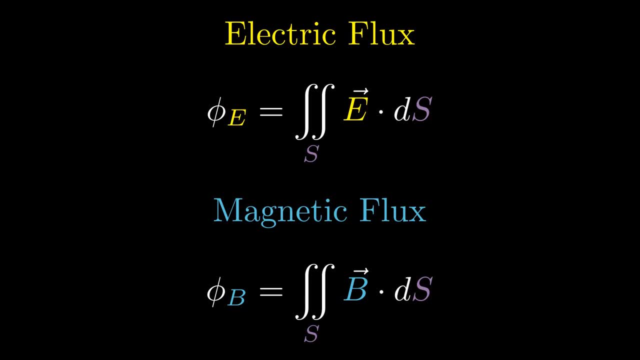 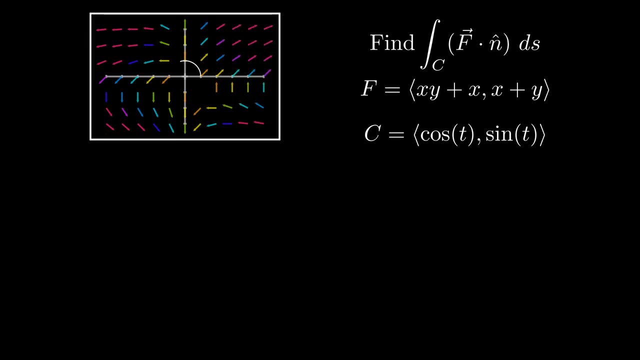 the surface. Let's try to calculate a 2 dimensional flux integral. Let's consider the vector field F is equal to, and let's say our curve is a circle with radius 1.. Let's try to find the flux integral over this curve of. 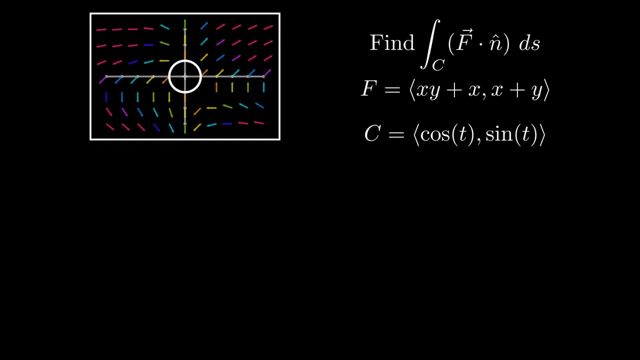 the vector field. So first we are going to parametrize this curve and it's a circle. so we get R of t is cosine of t and comma sine of t, And well, we need to find n hat. Well, what is n hat? 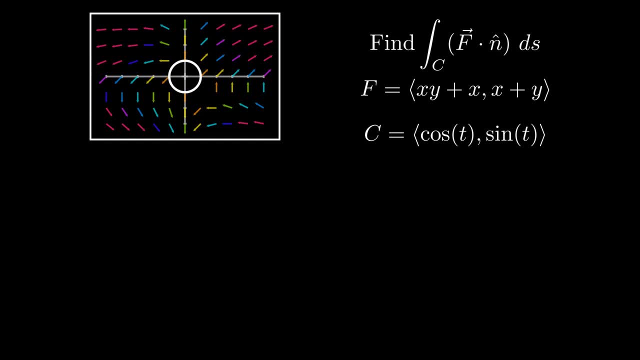 It's the normal unit vector which is perpendicular to the curve. Well, to do that, we just take the tangential vector and rotate it 90 degrees. Doing that, we get n. hat is equal to And. to calculate the flux, integral. if you remember, we have this formula and we plug. 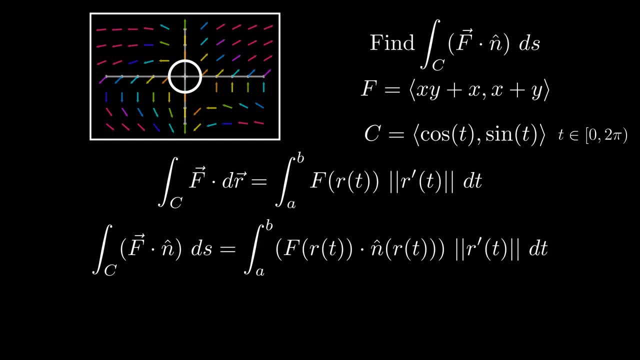 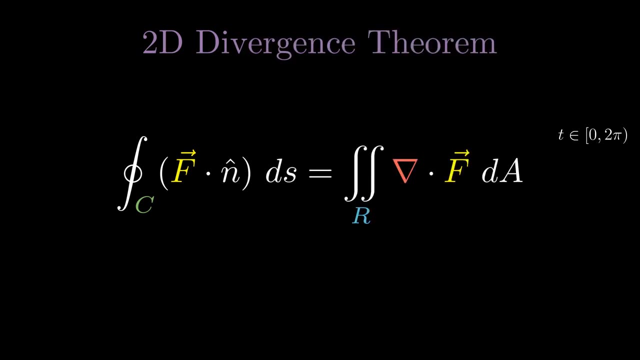 it and get an integral which evaluates to two pi. Now that we understand the concept of the flux integral, let's look at the statement for the divergence theorem, Theta: proprietary flux dot. M, presidente, E, Fi, V, C, r, z. integral of the divergence of F over R, Like curl divergence is another operation. 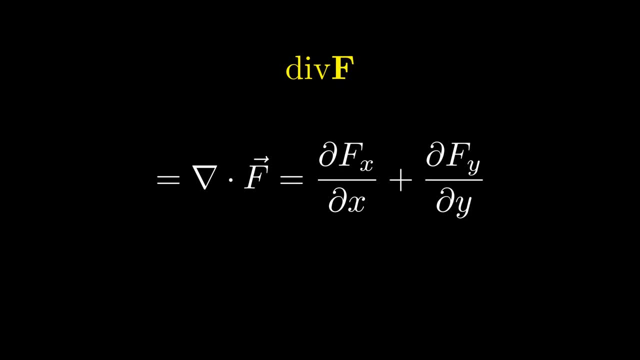 on vector fields. If you recall, curl measures the rotation of a vector field. On the other hand, divergence measures the outward flow of a vector field. Essentially, the divergence of a point tells you how much the vector field lines diverge away from that point. So for 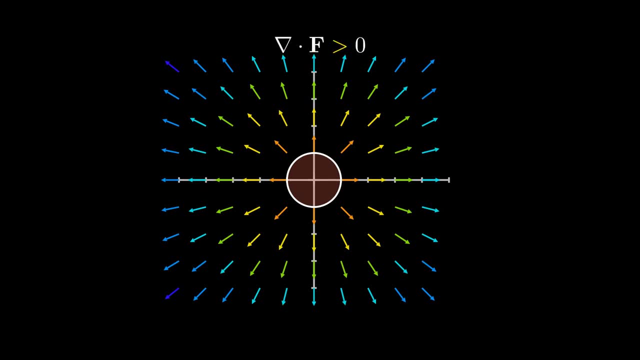 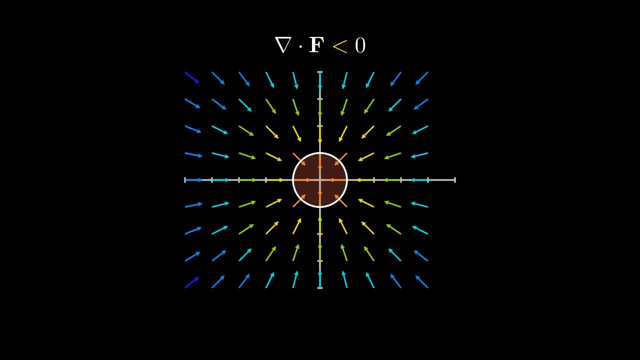 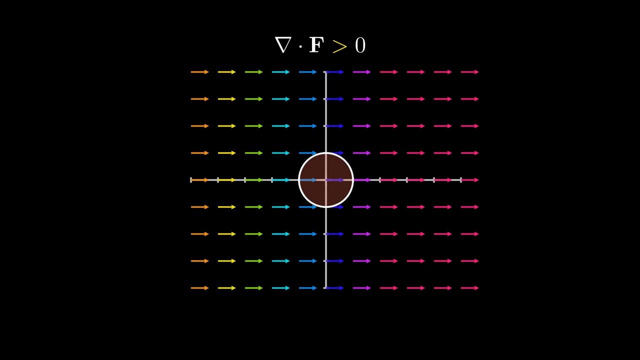 example, this region has positive divergence. It looks like the lines are coming out of this region which makes it positive divergence, essentially acting like a source for this vector field. And this region similarly has negative divergence. Positive divergence also occurs in fields like this. Let's go back to the divergence theorem, Our setup. 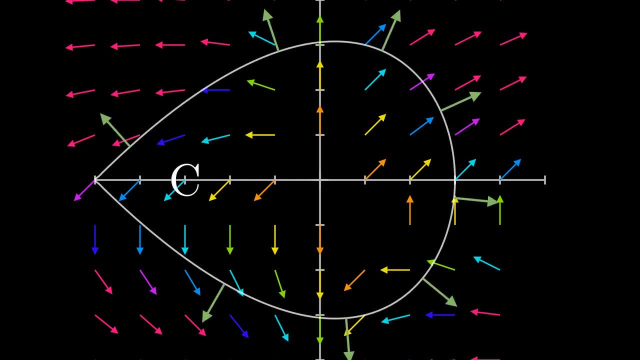 for the divergence theorem is pretty much the same as the one for Green's theorem. We have a vector field F and a closed curve C. Remember, this curve is oriented counterclockwise and it has to be closed. But, as we talked about earlier, we also have this normal unit vector function. 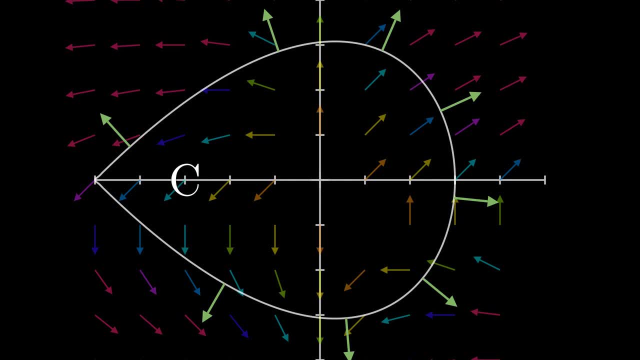 and had denoted in green, And in fact the proof is also very similar. If you followed along carefully, you probably already know where this is going. Since the flux integral is simply a line integral, like before, we can divide the curve into. 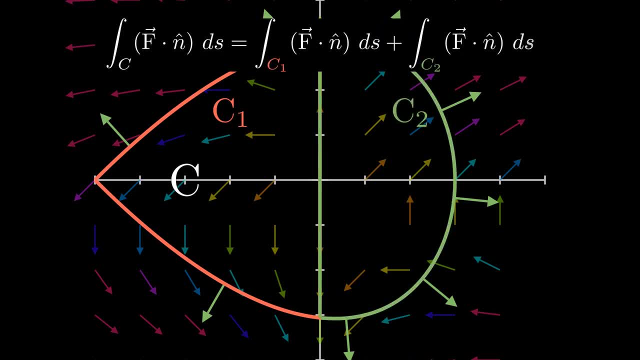 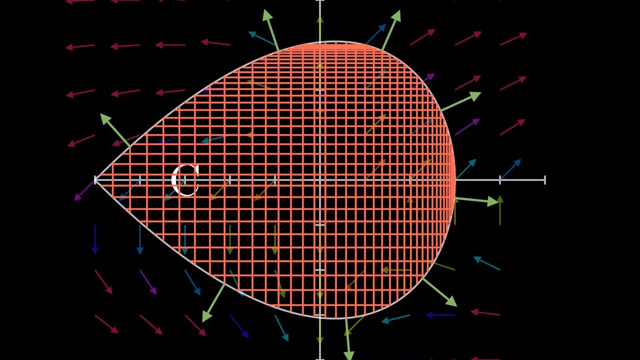 multiple pieces And the line integral of both of these pieces added up equals the line integral of the outside curve. As we go on, we can split the curve into many small pieces. Let's look at one piece. What does the flux integral around a really, really small curve? 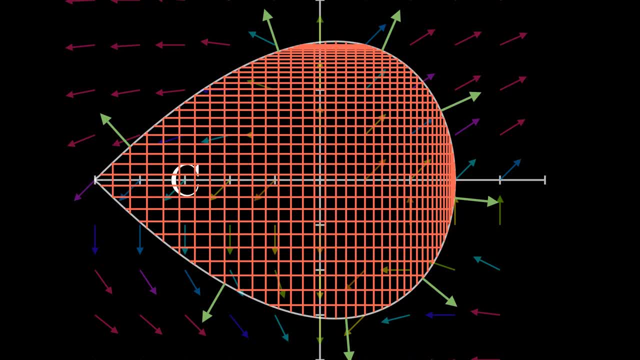 represent? Well, it's just the rate of flow through this curve. And since the curve is extremely, extremely small, it's approaching a point And the rate of flow through a point is just the divergence of the vector field. So we can approximate the flux integral of 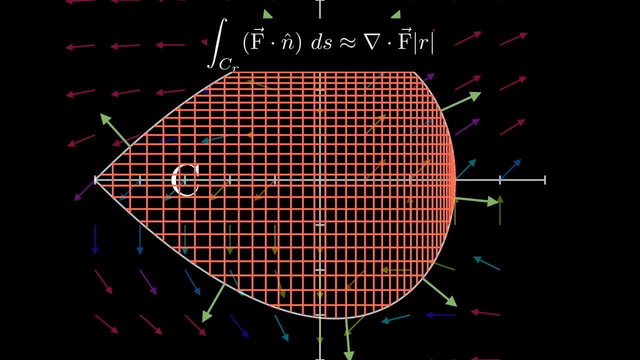 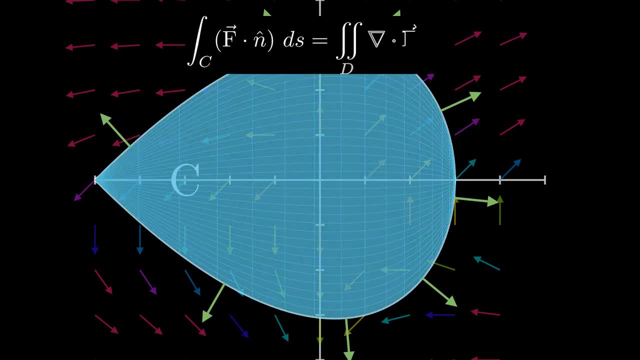 these small, small curves, using the divergence of our vector field. Thus, to get the flux integral of the entire curve, we simply sum up all the divergence inside this curve, which is just a double integral. So The outside curve can be equal to the double integral of the divergence of our vector field. 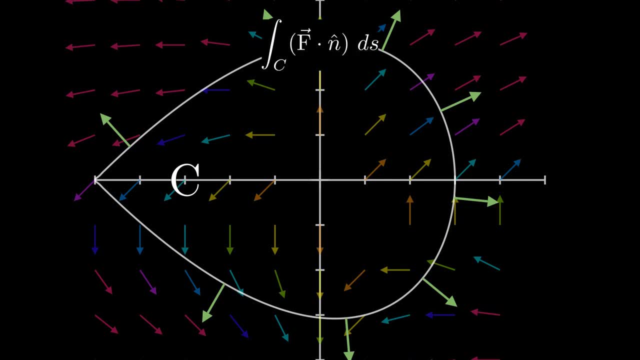 Let's try to look at this again. The curve can be split into different pieces, but the sum of the flux integral across these pieces is equal to the flux integral of the outside curve. So we can take advantage of this property by splitting our curve into many, many small. 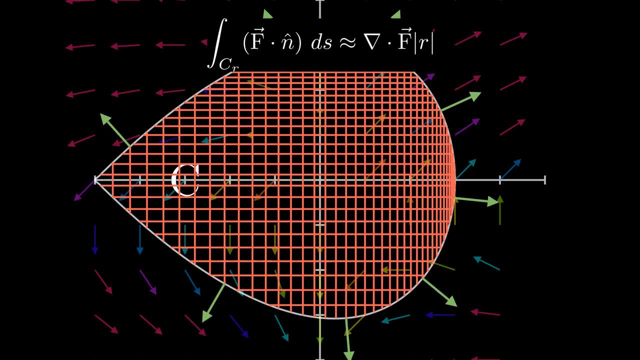 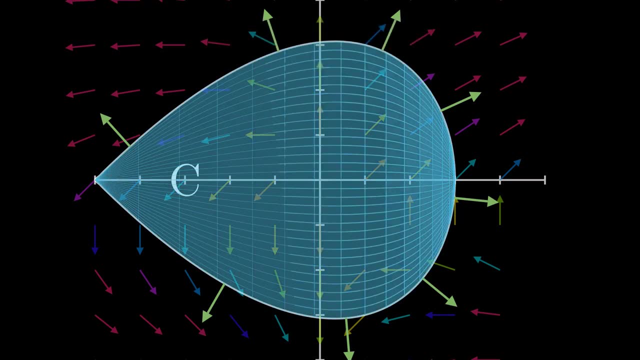 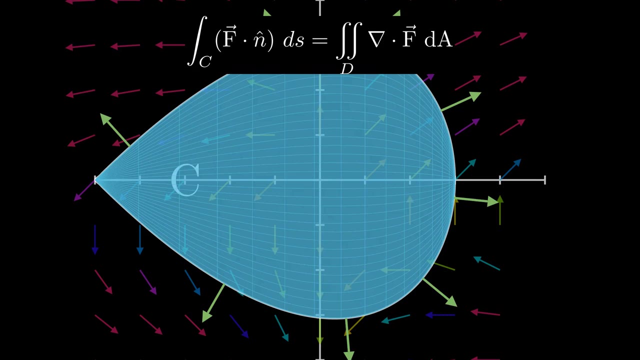 curves And, as I said before, as the curve gets smaller and smaller, it approaches a point. Moreover, the divergence becomes a better approximation of the curve, of the flux integral of the curve, as the curve gets smaller and smaller. Like I said, this intuition is quite similar to the ones for Green's theorem. You might 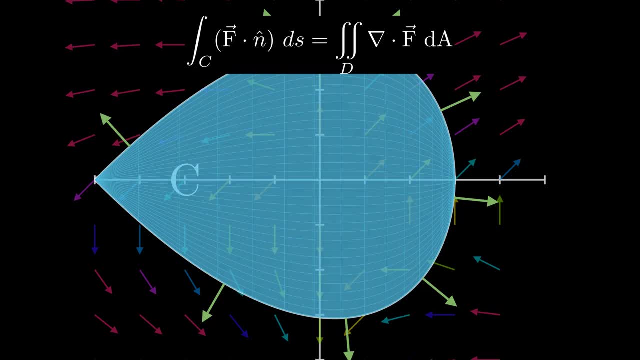 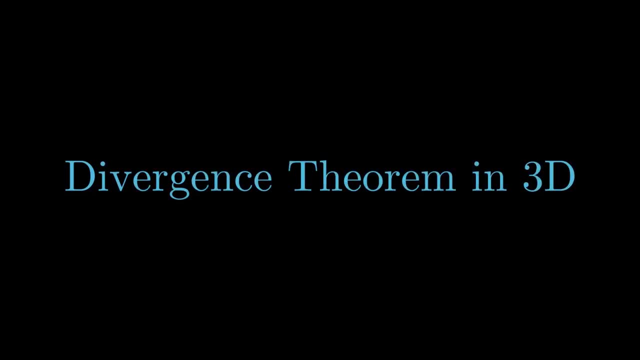 as well. watch my video on that. I've linked it in the description. But now let's talk about three dimensions: 3Dimensions, 3Dimensions, 3Dimensions- ignored If you aren't comfortable with the idea of integrating over a surface or a triple integral. 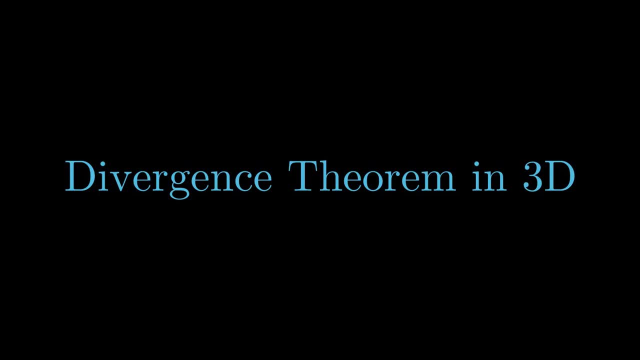 let's go quickly over what this means. When we talk about integrating over something, we are just summing up the value of the functions for all points within the region. So, for example, if you recall, a definite integral simply sums up all the values of a function between: 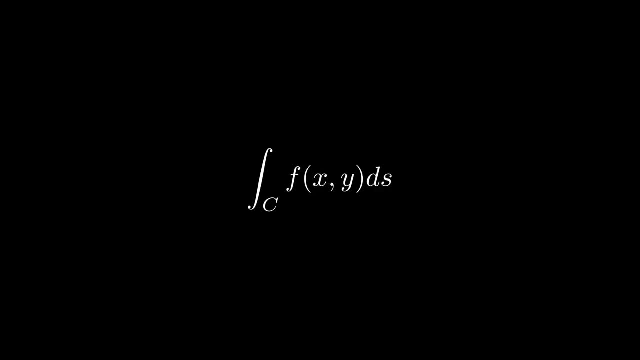 two X boundaries. Similarly, a line integral sums up all the values of a function over a curve. This is what MI экşîn comprehends: 1mHY3 volte 1mNOUm. We just家ut hold the 정 truth of the equation, because itясmies to aкийwa önкλη int0qurõs rjuçgä entre. 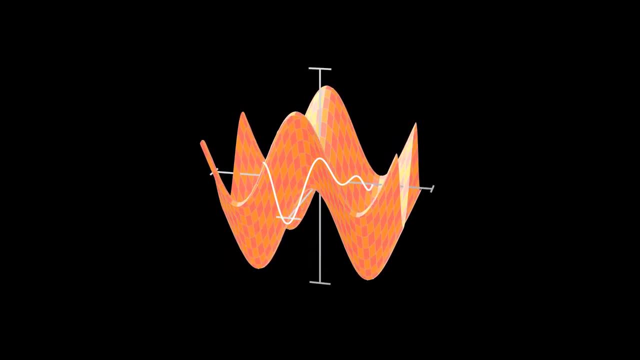 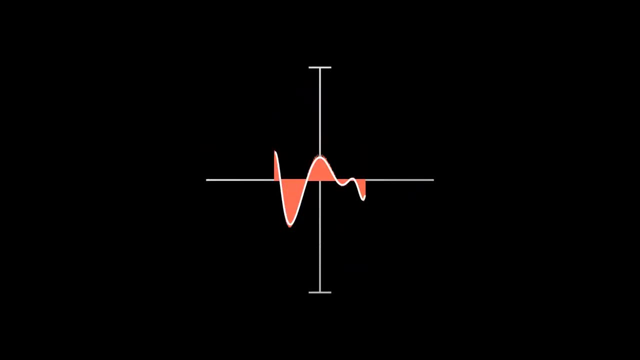 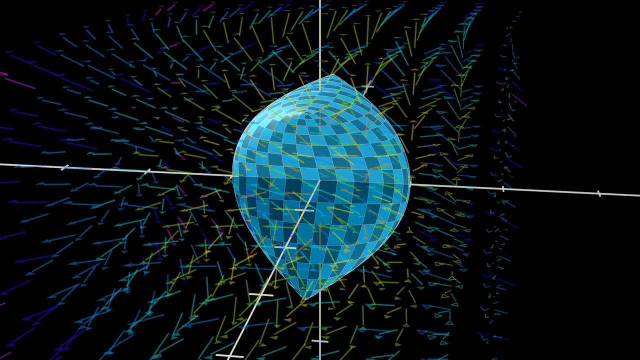 What I mean by this is that for every single coordinate pair on the curve I am just plugging in that value into a function and summing up its values. So a surface integral means summing up the value of a function for all points on a surface. 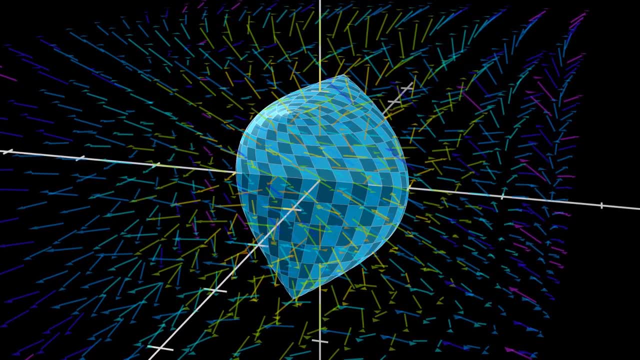 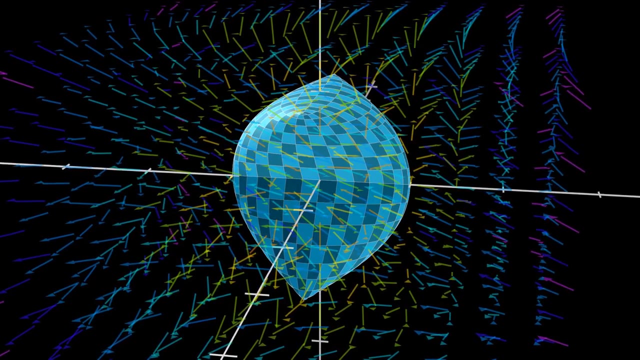 Thus, if our surface is in 3 dimensions, we would have a function that takes in 3 inputs. since our surface has points in 3 dimensions, A triple integral is the same thing, except, instead of summing up the value of a function for all points on a surface, we are summing up the value of a function for all points. 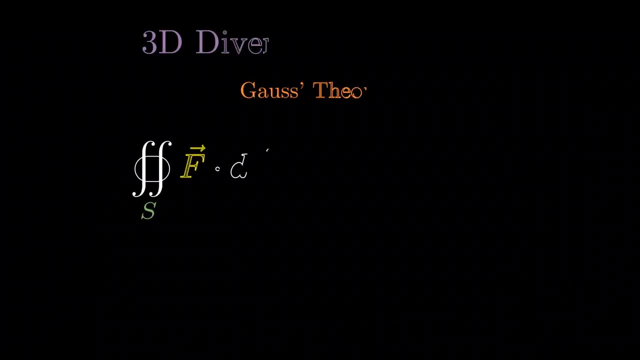 enclosed within the surface. Let's go back to the divergence theorem. The statement of the divergence theorem in 3 dimensions goes as follows: The flux integral over a closed surface S is equal to the triple integral of the divergence of the vector field over the region within. 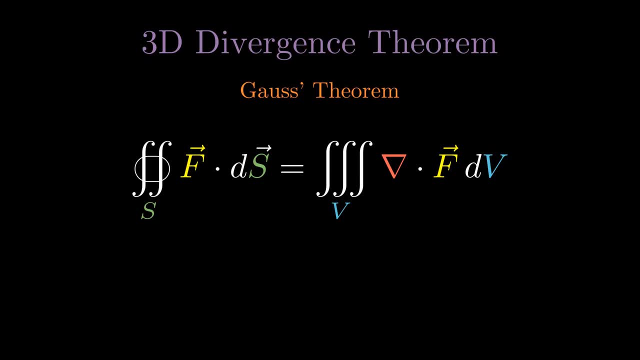 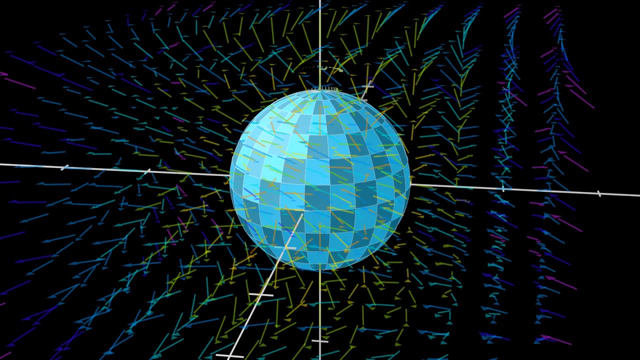 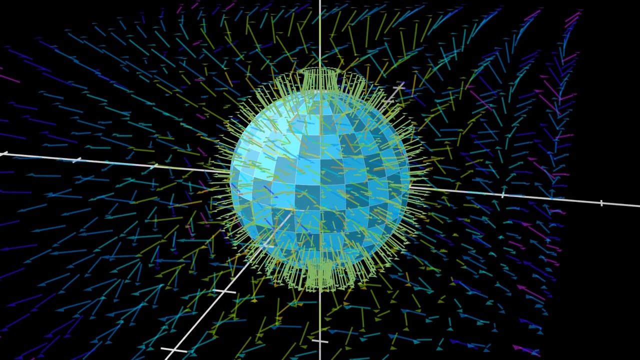 the surface. Let's look at our setup. Instead of working in 2D space, we are working in 3 dimensions. There is a closed surface, S, which I am going to use a sphere for for simplicity, and V is the space enclosed within the surface. F is the 3 dimensional vector field. 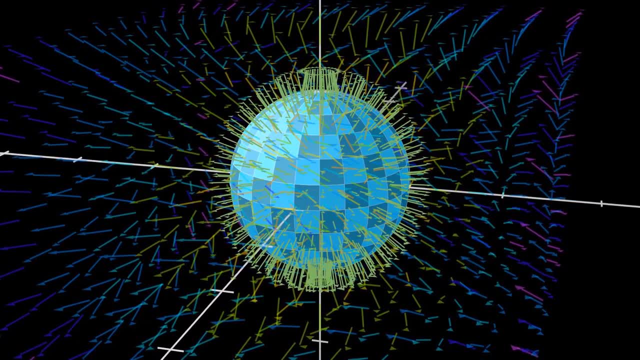 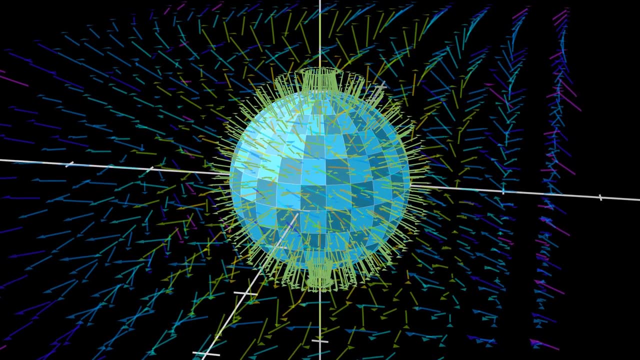 The last part of our setup is a vector function that gives a vector perpendicular to the surface, like the 2 dimensional version. If you recall, this is n-hat. I am denoting n-hat by green. You probably know where this is going again. 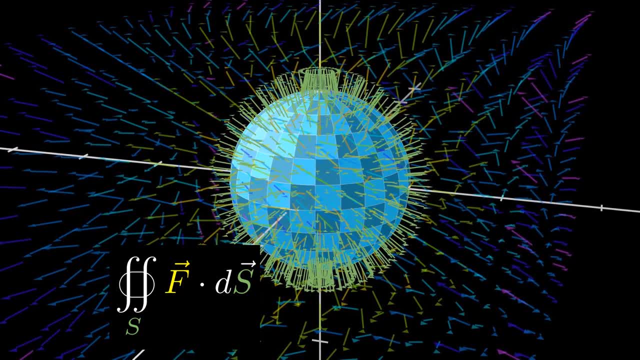 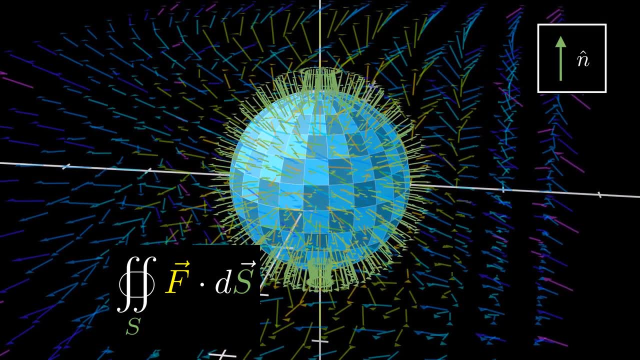 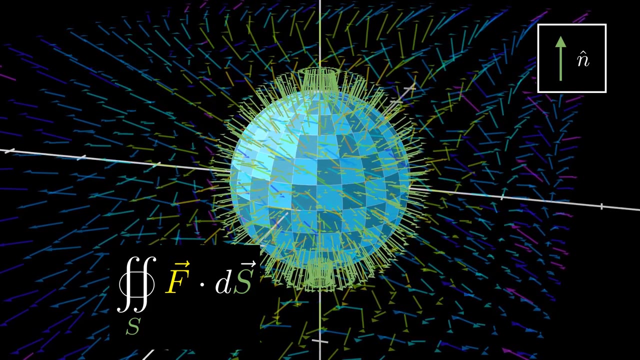 A surface integral of a vector field is flux in 3 dimensions. so we are measuring the flow rate across an entire surface, similar to the divergence theorem in 2D, As we discussed before. the divergence of a vector field gives the flow rate at a point. 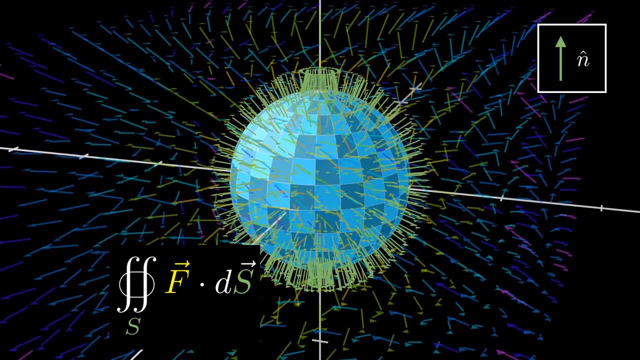 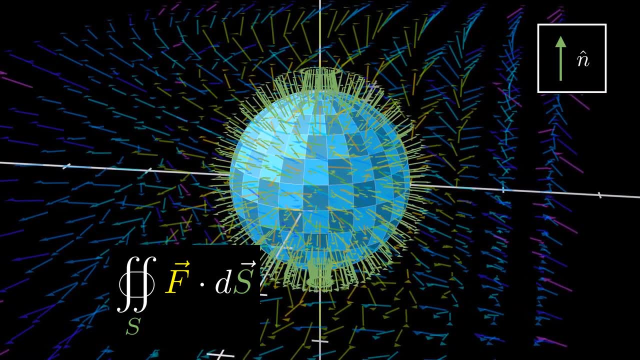 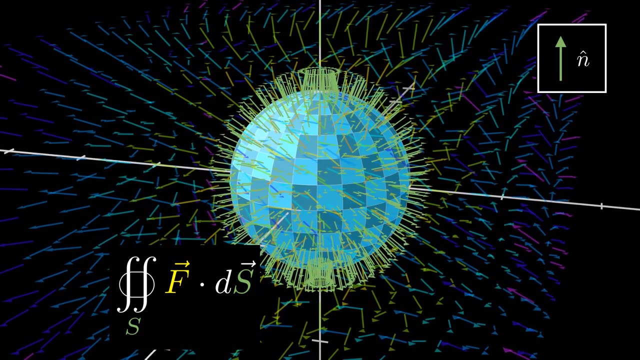 And instead of considering really small bits of area, let's consider what we get when we sum up the tiny little bits of volume. Since we are integrating over a 3 dimensional space, we use a triple integral. The triple integral gives the total output flux around V of F, No three dimensions. 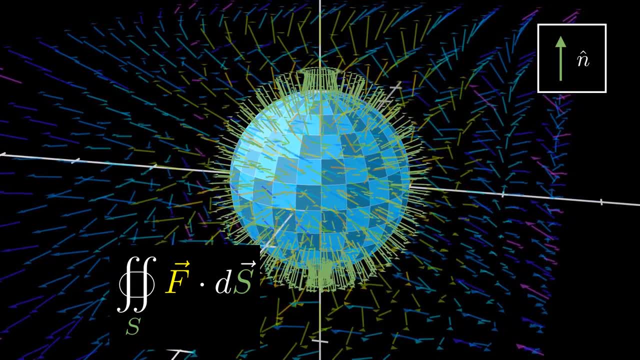 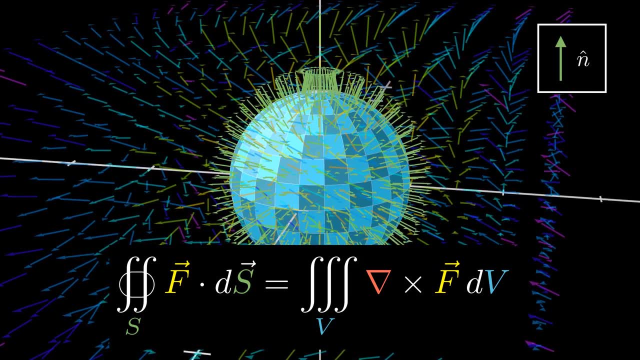 Thoughts in the background. Also very upsetting When you write a total gyram of cross determ kinets in 3 dimensions and where a note the keyword around- That means it's the same as the flux over the surface S. This is the divergence theorem. It relates a flux integral in three dimensions with a triple 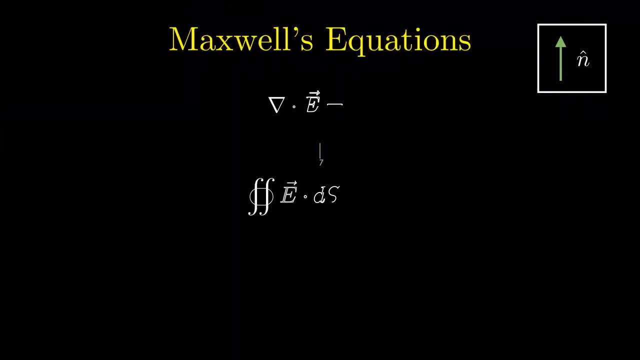 integral. The applications of divergence theorem are many, but one key application is in Maxwell's equations, when you can convert them between integral form and point form. But that's for another video. Thank you for watching.